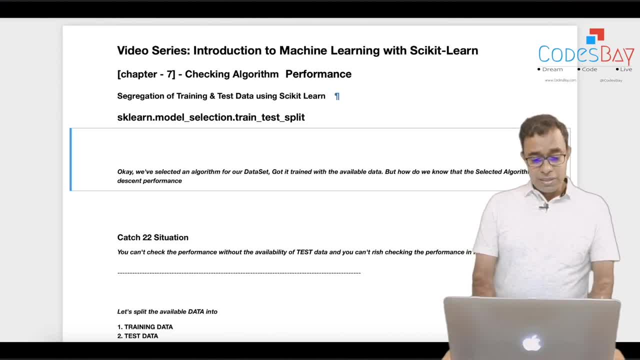 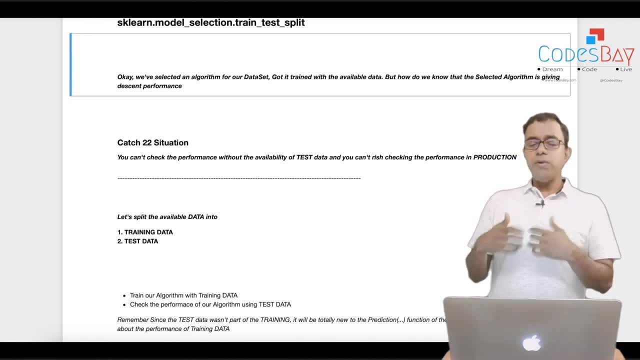 we have to understand the algorithm performance. How do we do it? So okay, we have selected our algorithm, got it trained with available data, but how do we know that the selected algorithm is performing better than other algorithms? Now, it is a catch-22 situation. You know why? Because 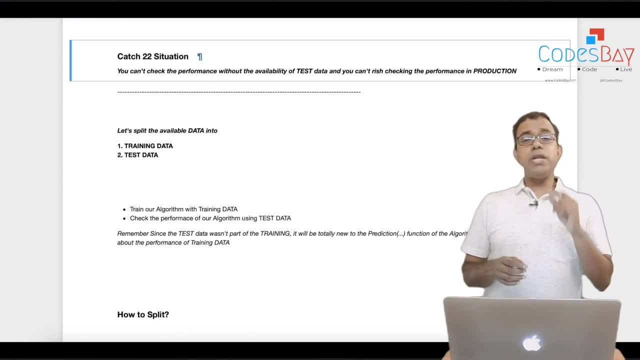 you can't check the performance of your algorithm with training data set. You need some new data and unseen data to be able to judge the performance of your algorithm. So when you get a data set, you don't get testing data set, you just get a data set right and you cannot check the performance. 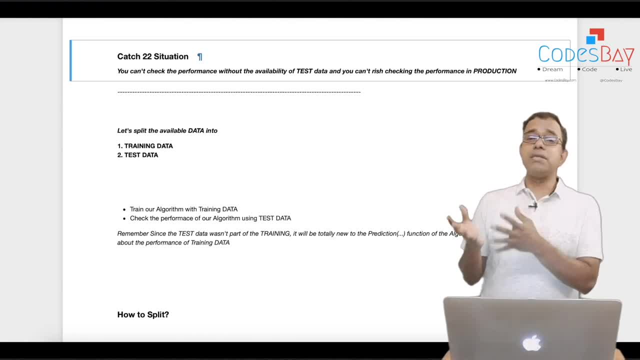 of your algorithm in production. Okay, deploy it in production, we will see, because you know what. if you judge your algorithm with training data, with the same data set, then you cannot get the data you have provided for training purposes. most of the time, your performance will be decent- Okay, it's only when we get unseen data. the real performance of the algorithm is. 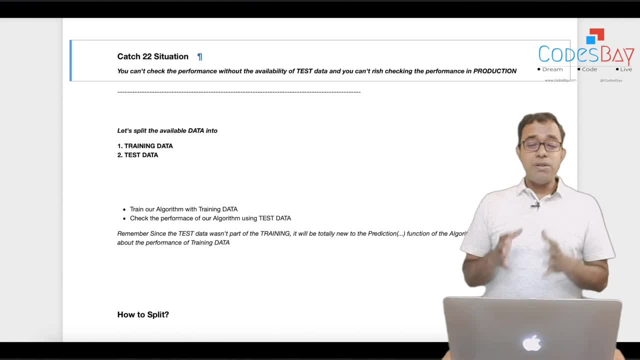 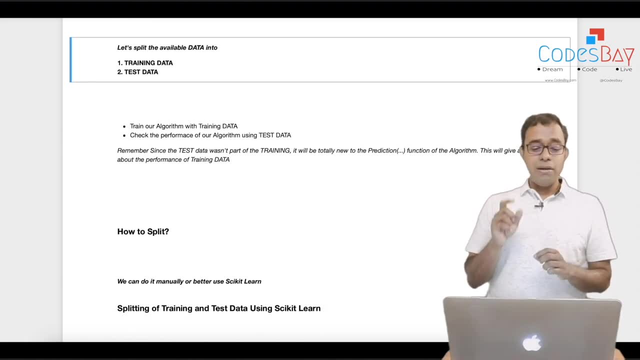 being checked. So now it's a cat's 22 situation, and the solution to this catch 22 situation is we have to split our available data into two set called training data set and testing data set. So what we will do is that we will train. 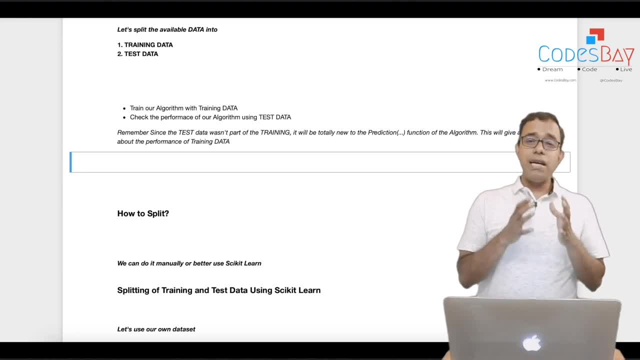 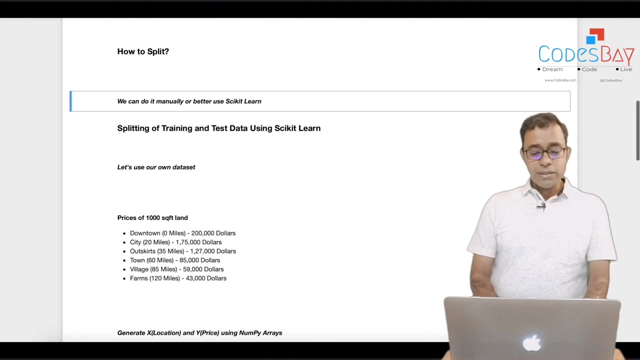 with training data set and we will test our algorithm with testing data set now. since we are not providing testing data set as part of training our algorithm, the testing data set will be considered as new as unseen data, as any production data. okay, now the question arises that how to split these data now? there are two ways of doing it. we can do it manually, of course. 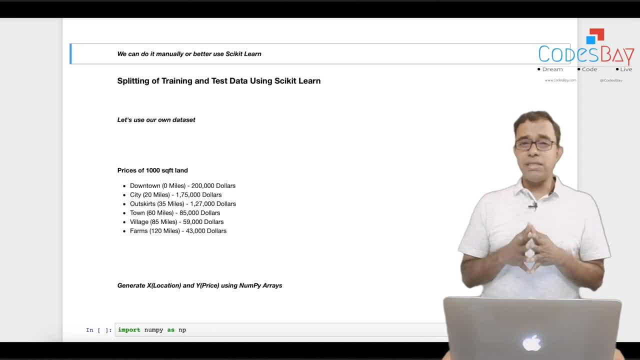 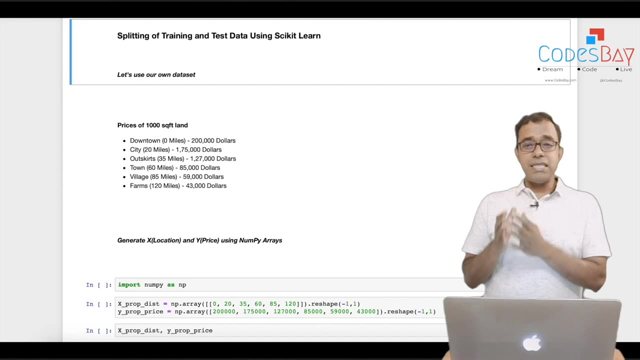 it will take more effort and it may not be a judicious decision also, so let's use the functionality provided by scikit-learn to split data into training set and testing set. now, to understand this splitting of data into training set and testing set, let's generate our own data. 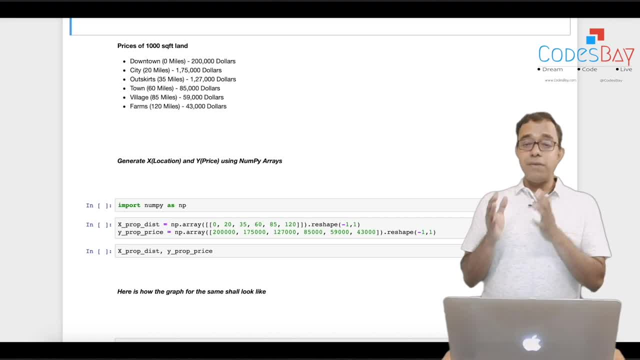 set first. so this is the data set which i have used in chapter 6. i will highly recommend you to go ahead and see how this data set was used with linear regression algorithm. now here is how the data looks like. this data is all about the price of 1000 square feet land. 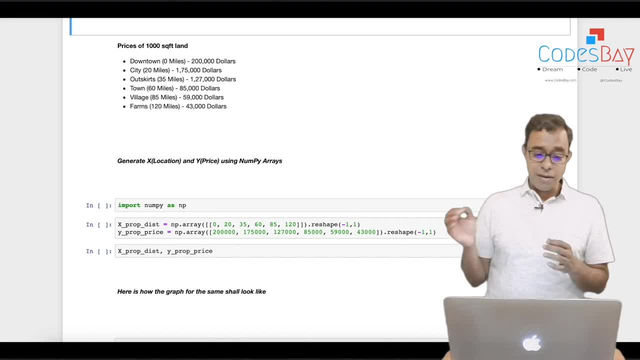 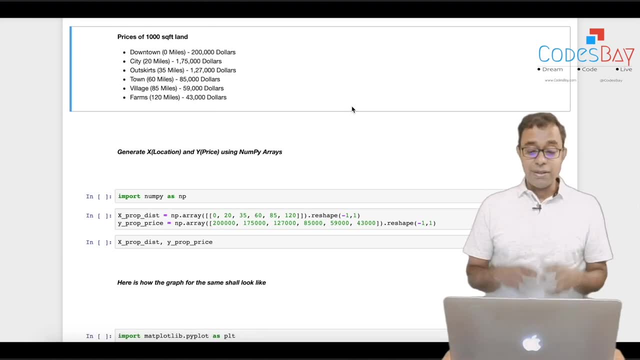 at various locations from downtown and far away from that. so at downtown it's two hundred thousand dollar. city, 175, outskirts, 127, town which is 60 miles from downtown, 85, village, 59, a farm, which is 120 miles from downtown, it's forty three thousand dollars. now let's generate our x-axis. 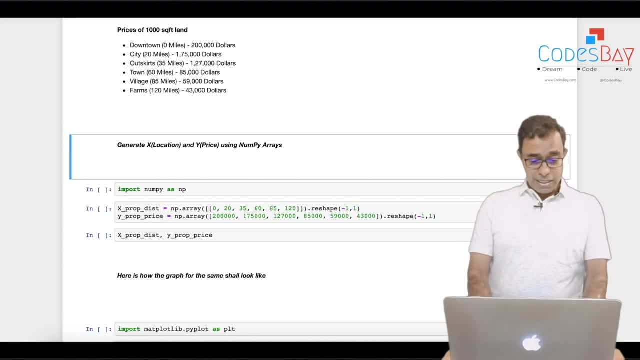 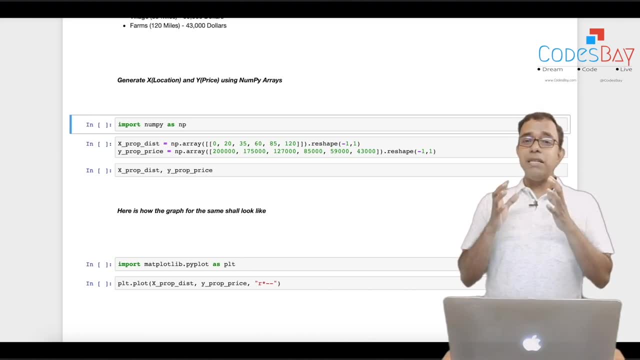 and y-axis, x will be location and y will be the price. okay, now we will generate numpy over here. we will not use python arrays, because numpy is what we use for machine learning in python. okay, so if you are not comfortable with numpy, just go back and see one of my video in this particular series, where 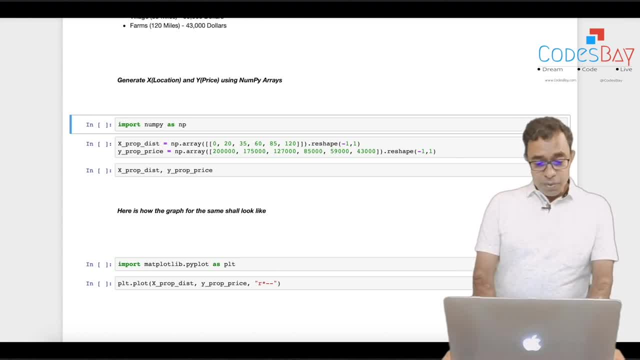 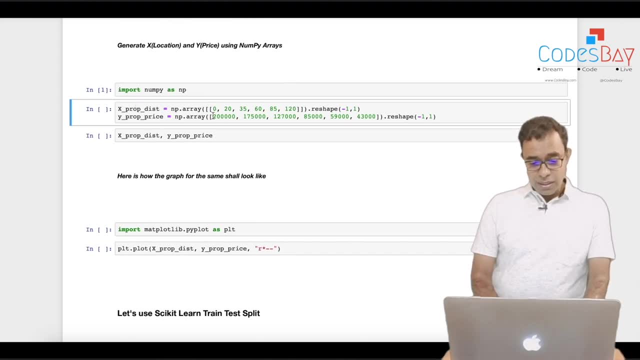 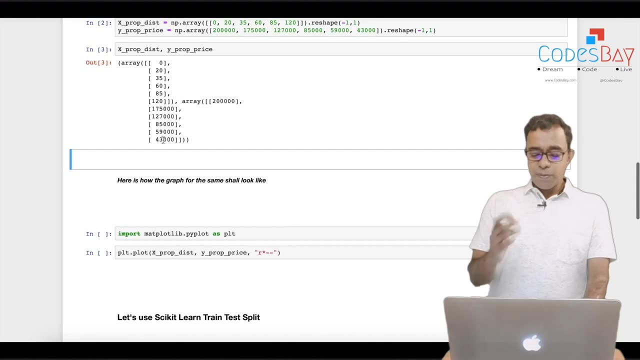 i talked specifically about numpy, so i will import numpy as np. i will create x prop distance and y prop prices. so this is miles from the downtown and these are prices. and here is how my numpy arrays looks like: this is x, this is y. let's plot the same also. so let's plot the same using matplotlib dot pi. plot again: i have 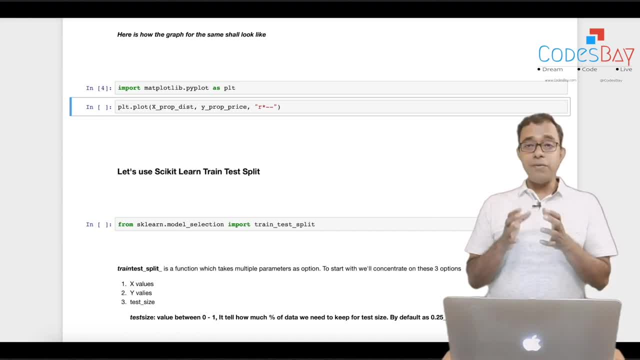 also explained how to use matplotlib piplot in one of the video in this particular series. i will highly recommend you to go ahead and look into that video if you are not comfortable with matplotlib dot piplot. so here is how our plotting looks like. okay makes sense, it's. 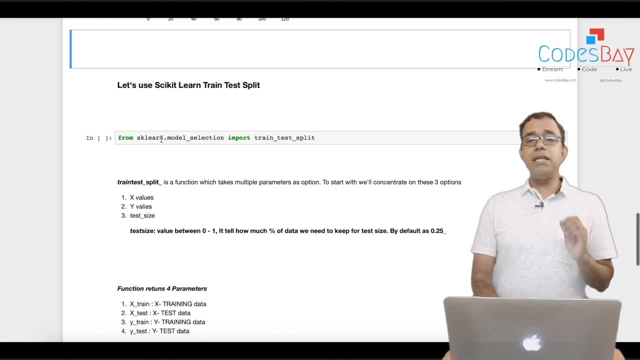 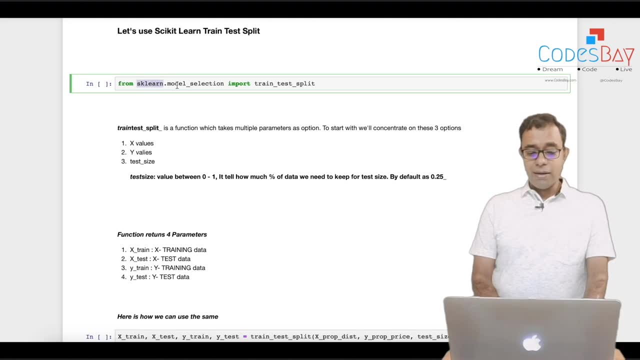 of linear relationship. now let's use train test split from the scikit-learn to split the data. to use this, we will have to use scikit-learn model selection import train test split. now this train test split is a function, it's not an object. remember, it's a function. now this function takes: 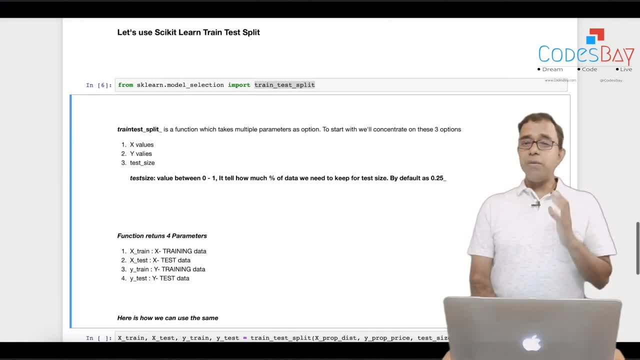 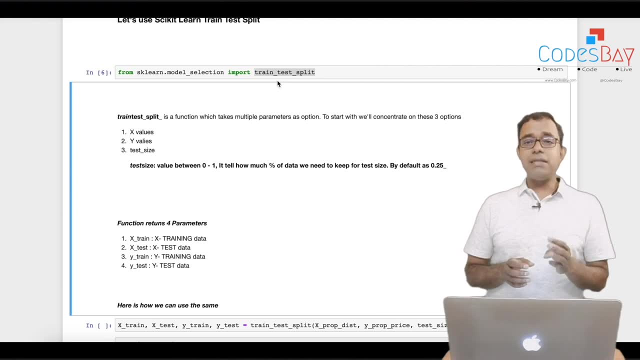 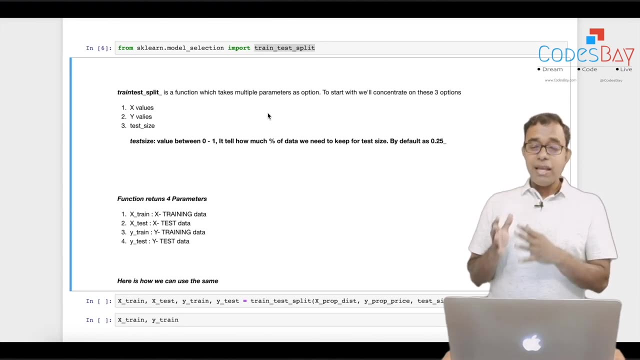 multiple parameters. you can provide multiple parameters, some of which we are going to talk about now. okay, so to start with, let's concentrate on these three parameters. i will talk about another parameter at later part of this video. now let's see these three parameters, so x and y. 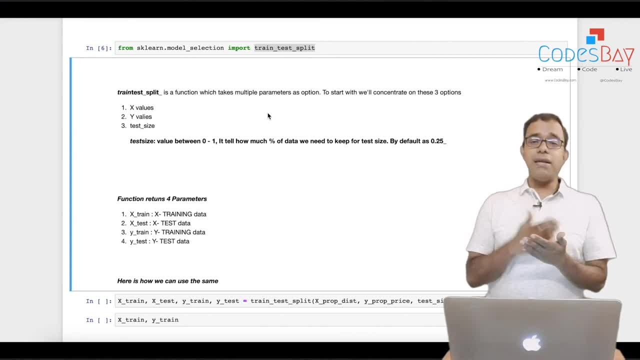 values are mandatory, which you need to be splitted into training data and testing data. x and y you have to give now this parameter is interesting- test size. this parameter takes a value between 0 to 1, which is equivalent to 0 percent or 100 percent. 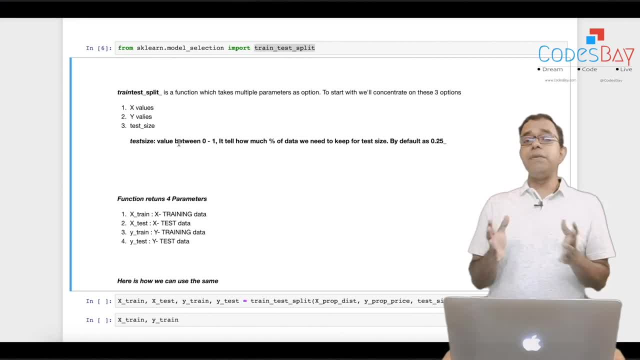 it tells you about how much data out of the available data should be kept aside for testing purposes. by default, the value is 0.25, which means that if i have 100 samples, i should keep aside 25 samples for testing and i will give 75 samples for training purposes. so if i set it to 0.10, 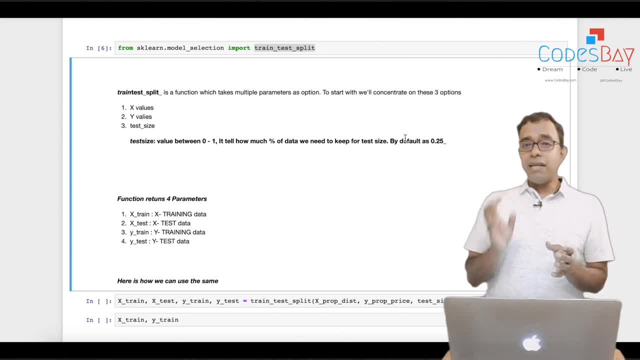 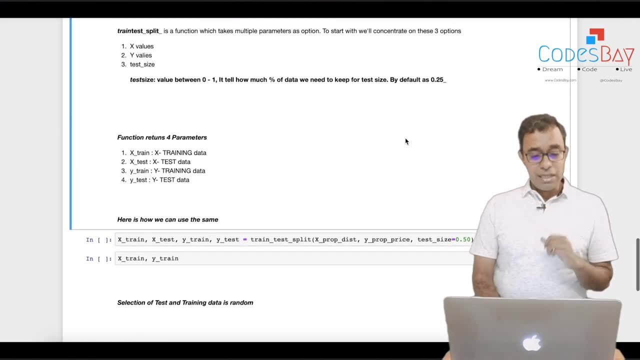 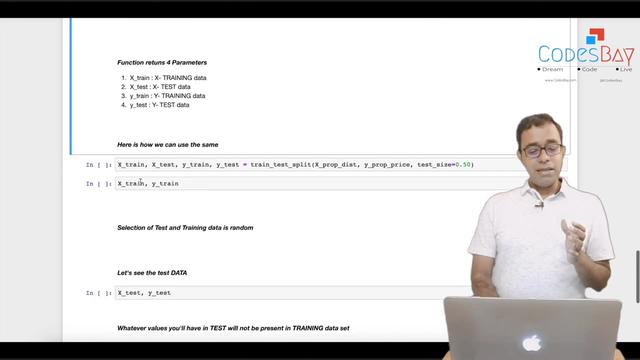 it means that it will keep aside 10 samples for testing and it will give 90 samples for training purposes. so let's understand the return values. it returns four parameters, okay: x train, x test, y train, y test. these parameters are self-explanatory. x train means x value for training, x test means x value. 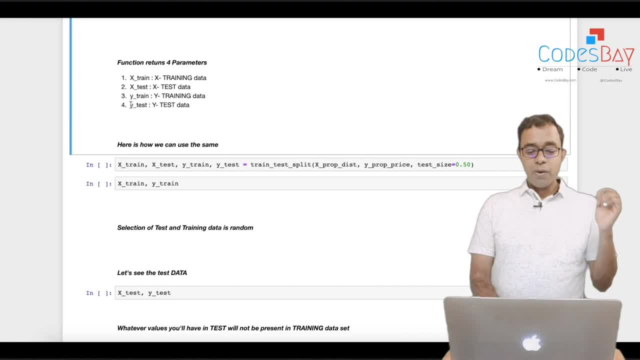 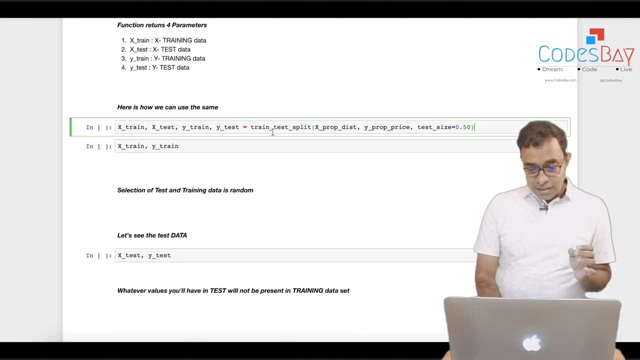 for testing. y train means y value for training, y test means y value for testing. to train the data, we will use x train and y train. to test the data, we will use x test and y test. now let's see how we can use this particular function. we'll call this train test split function. we pass x, y and the. 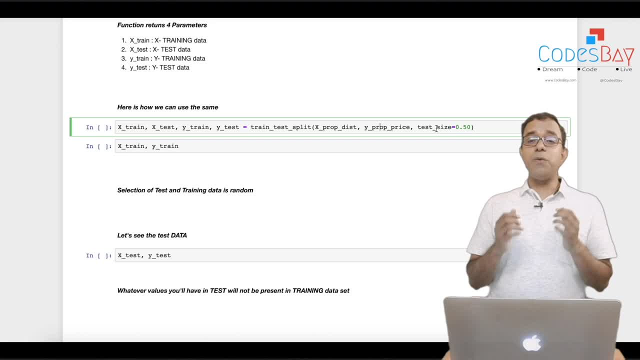 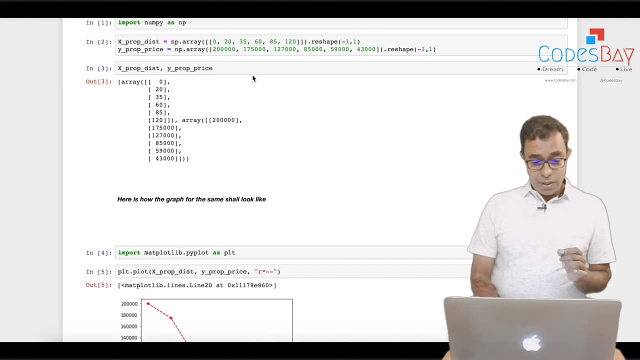 test size, i am passing 0.50, which means that i want 50 percent of the data to be kept aside for testing and rest 50 percent of the data for training purposes. i run this code. let's see how the output looks like. remember i have six data set right: one, two, three, four, five, six out of six. 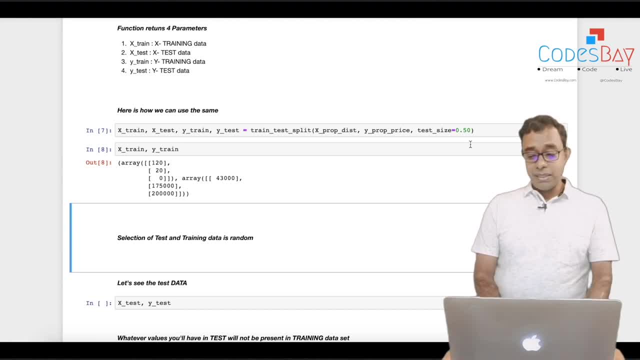 and i have two, three, four, five, six out of six. so this is the output which is given to me as a training data set. these three are randomly selected and if i call this function again every time, you can see that the values will change. it will give you different values and this randomness is good. 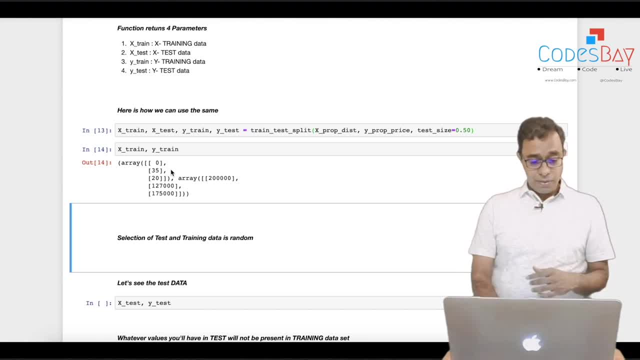 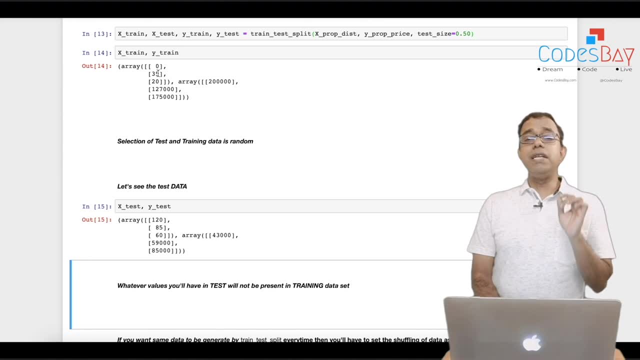 you don't want to sequentially take first few data for testing, last few data for training, or vice versa. okay, so let's see test data. okay, so whatever will be there in a training set will not be present in the test set. so let's see test data. okay, so whatever will be there in a training set will not be present in the test set.